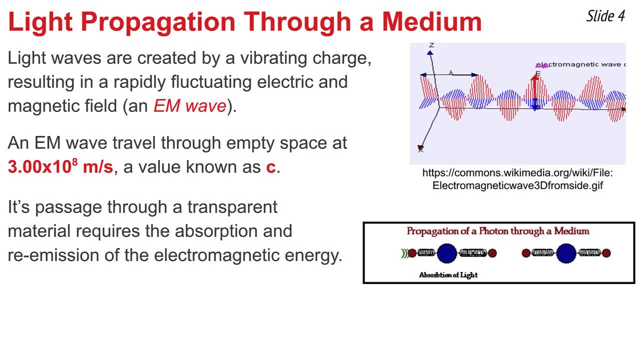 it travels through a transparent material, the atoms of that material absorb its energy, causing electrons in the material to vibrate rapidly, before finally re-emitting its energy as a new electromagnetic wave. This process of being absorbed and re-emitted continues from particle. as the light wave makes its passage through that transparent material, It travels from particle. 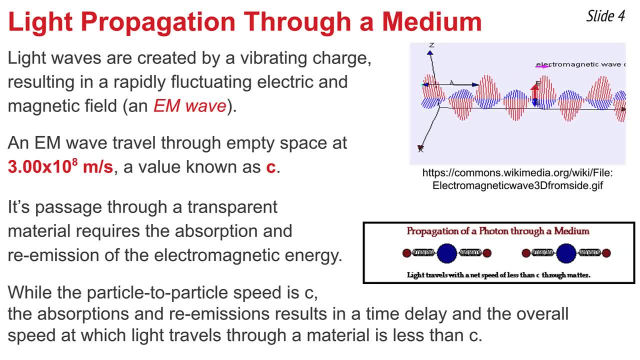 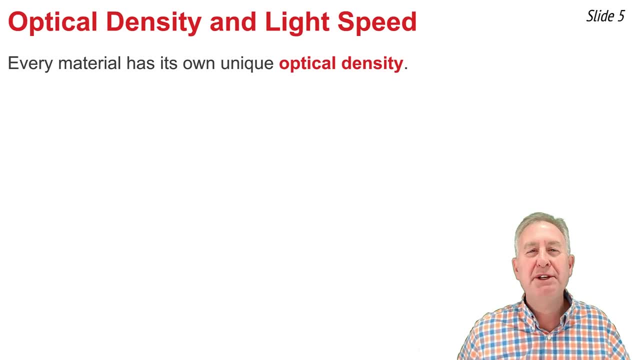 to particle at a speed of 300 million meters per second, but it's the absorption and re-emissions that result in a small time delay, causing the overall speed of a light wave through a transparent material to be something less than c 300 million meters per second. Every material has its own. 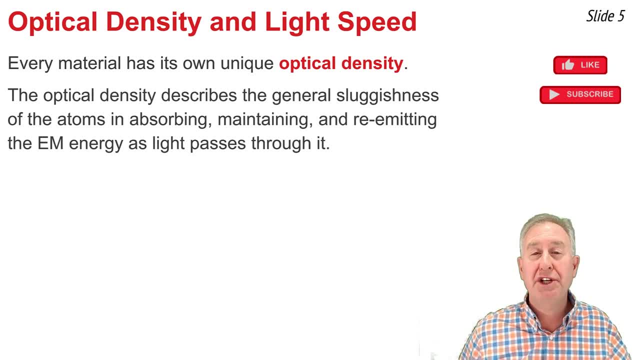 unique optical density. Optical density refers to the general sluggishness of the atoms of the material as it absorbs, maintains and re-emits the electromagnetic energy as the light wave passes through it. The greater that the optical density of a material is, the slower that light. 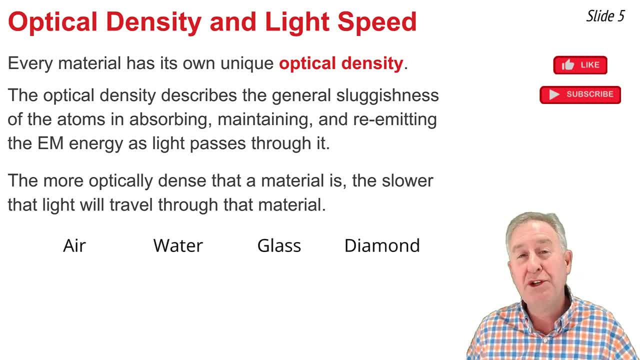 will travel through that material. Here are four materials, arranged in order of their optical density, with air being the least optically dense and diamond being the most optically dense. Given our rule about optical density and speed, we would reason that light will travel fastest through air. 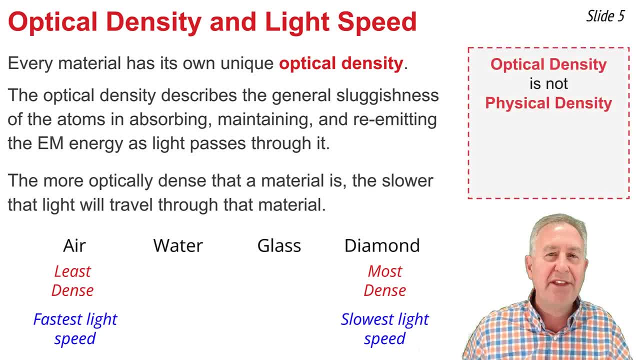 and slowest through diamond. Optical density is not the same thing as physical density. You may have learned about physical density as the mass per volume ratio in another science class. Optical density is not mass per volume. Instead, it simply refers to the general tendency of the atoms of the material to get in. 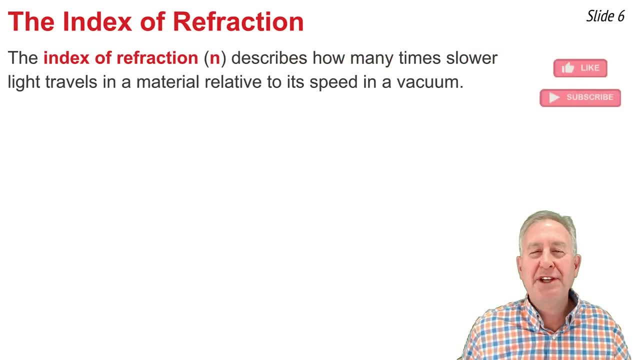 the way of light as it passes through it. Just as every material has its own unique optical density, so does every material have its own unique index of refraction value. The index of refraction value is the individual index of refraction value. Each Arai, Nazi and Nazi. 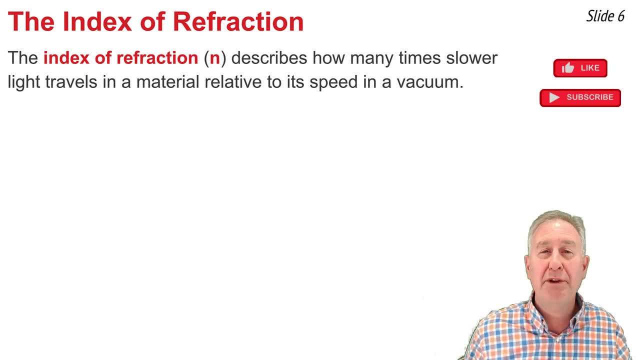 value refers to how many times slower that light will travel through that material than it does through a vacuum. The equation for n, the index of refraction, is: n equal c divided by v, where c refers to the speed of light in a vacuum 3 times 10 to the 8th meters per second and v refers to 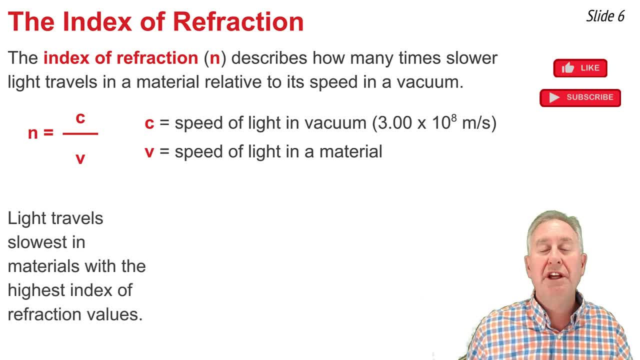 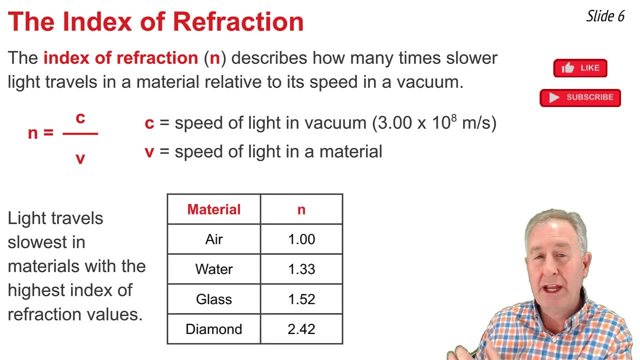 the speed of light within that particular material. The rule is that light will travel slowest in materials that have the greatest index of refraction value. Here are the four same materials we discussed earlier- air, water, glass and diamond- and their index of refraction. 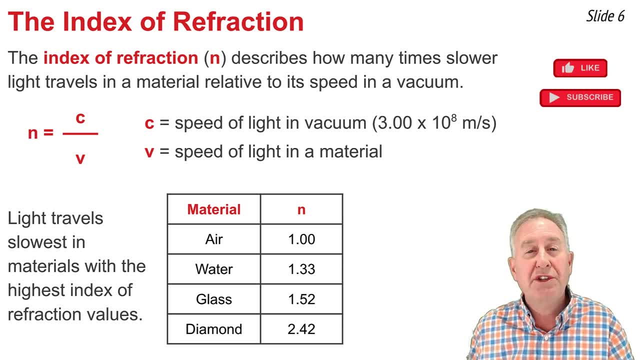 rounded to the second decimal place is listed. You'll notice that air, the least optically dense material, has the smallest index of refraction and diamond, the most optically dense material, has the largest index of refraction. We can take these values of n and substitute it into the. 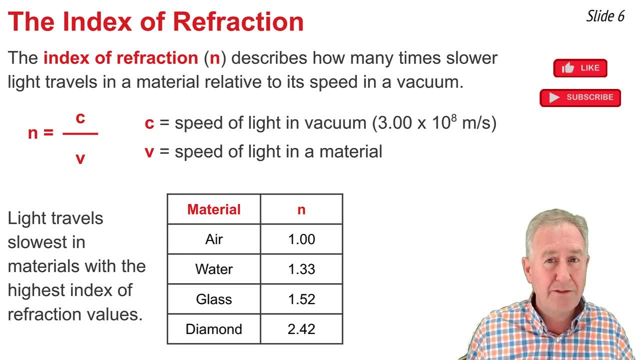 equation and solve for v, v the speed of light in each of these materials. The equation will have to be rearranged to: v equals c divided by n. then we substitute in the value of n and we'll get these values for the. 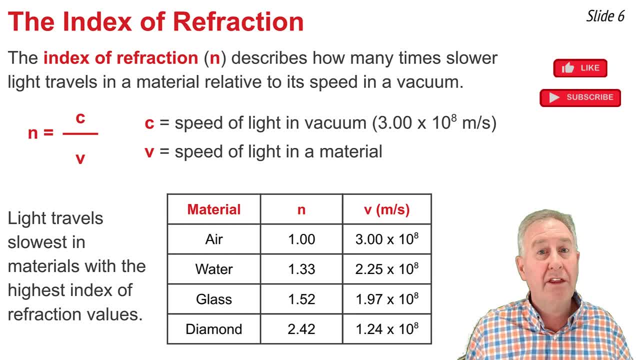 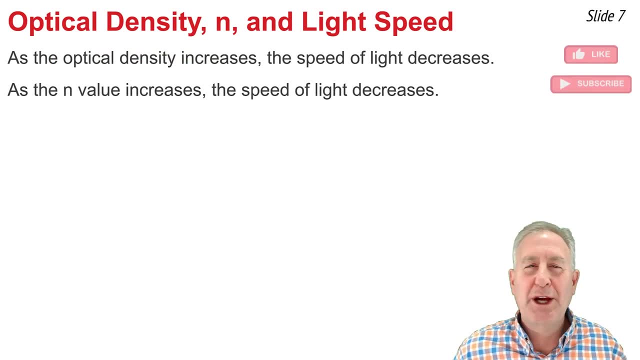 speed of light in each of the materials. You'll notice that air, the least optically dense material, the one with the smallest n value, has the highest speed, and diamond, the most optically dense material, the one with the largest n value, has the lowest speed of light. Here is a summary. 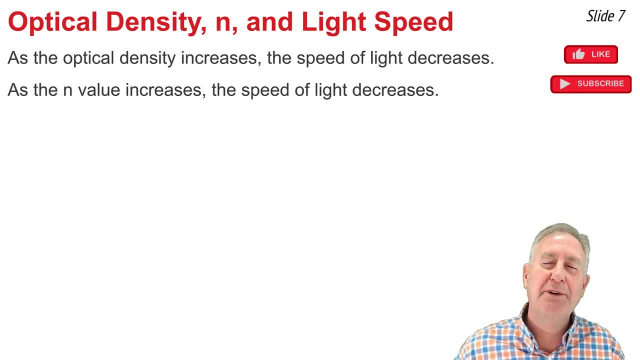 of the rules. See the video description for more information. The relationships between optical density, index of refraction and the speed of light. Optical density and the speed of light are inversely related, And the index of refraction of a material and the the speed of light in that material are inversely related. 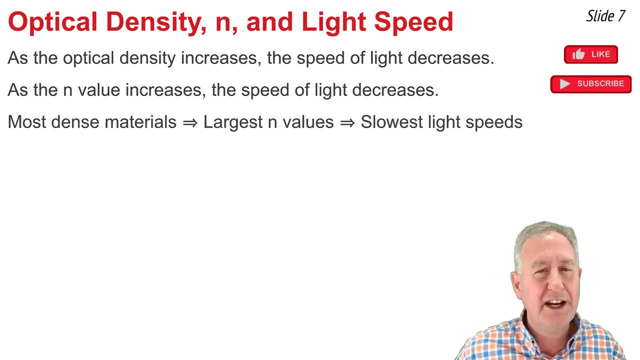 are. thus we could reason that materials that are most optically dense have the largest index of refraction value, and light travels slowest through those materials And materials that are least optically dense. refraction values in light travels fastest through those materials. The 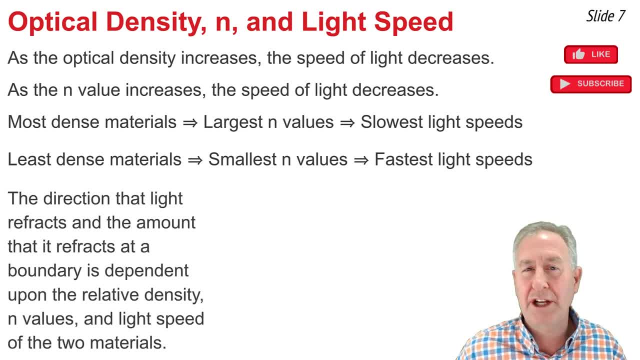 importance of this information is that it helps us to make a prediction of the direction in the amount of refraction that occurs at a boundary as light passes across the boundary, For the direction and the amount of refraction depend upon the relative values of the optical density, the index of refraction. 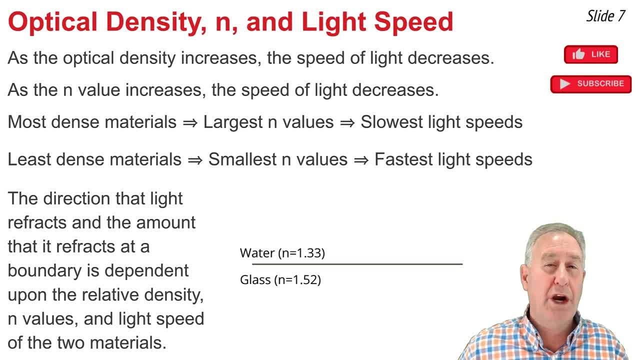 and the speed of light. For example, let's consider a light ray passing from water into glass. The index of refraction of glass is greater than that of water, and so when light crosses the boundary from water to glass, it will slow down And the 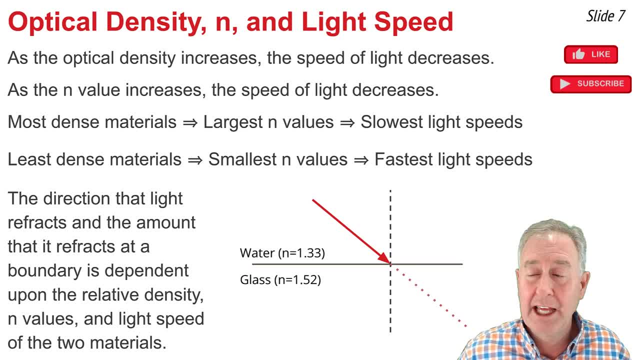 slowing down means that light won't travel in a straight line. It won't follow the dashed path here on the diagram. Instead, it refracts in one of two directions. Either refracts so that the light ray in the glass is closer to the